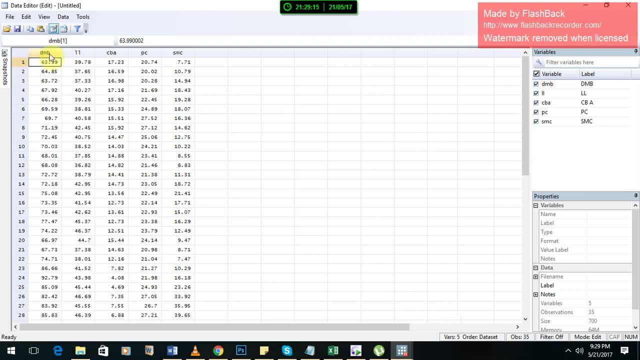 your variables with your data. In that way, your variables will be shown up over here, And remember that your variable should not contain any space, because Stata might not take such variables with the space. So after pasting them over here, now go back to the Stata. Now there are two ways: Either you 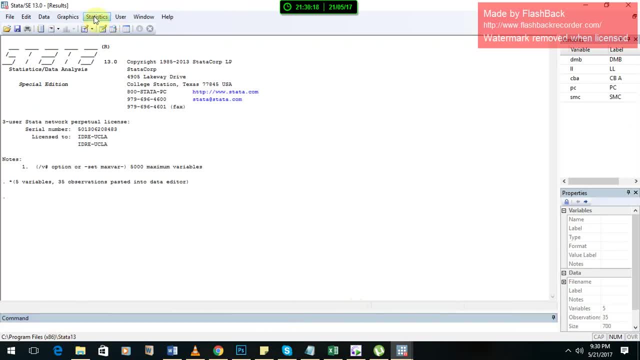 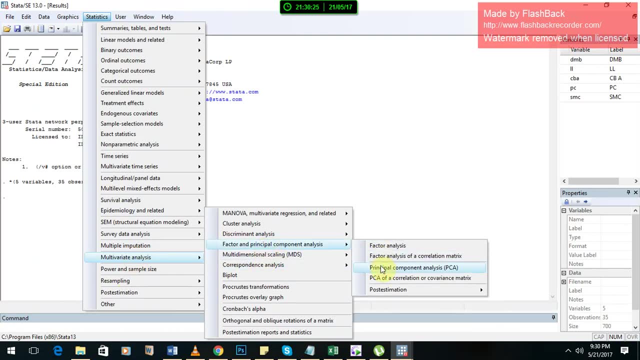 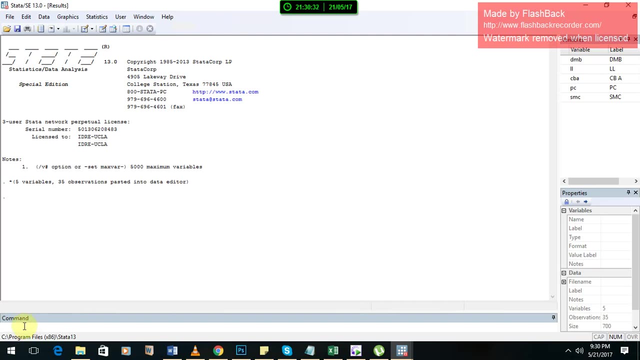 can use the command of PCA or you can go to the statistics: multivariate analysis, factor and principal component analysis and PCA. If I just clicked it it will automatically run the results, But I'm going to show you how to run through it with the command Write. 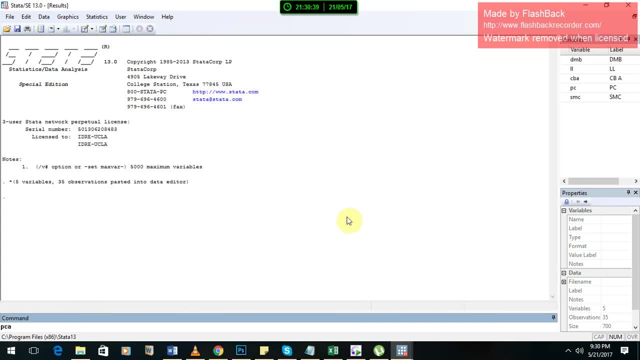 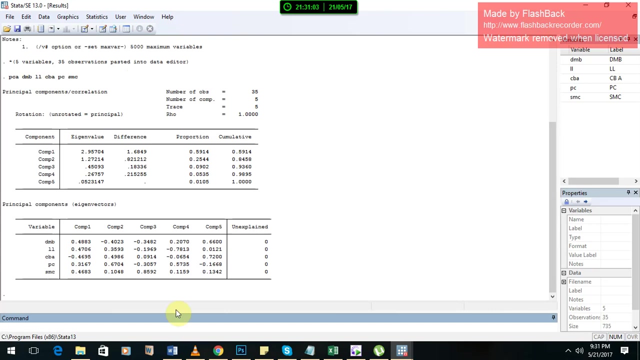 PCA in the command section Space and the variables names are shown over here. You can see them over here or you just can write them: DMLL, Sorry, DMLL. Space, CBBC, Space, SMC. Now just press enter And it will run the results. 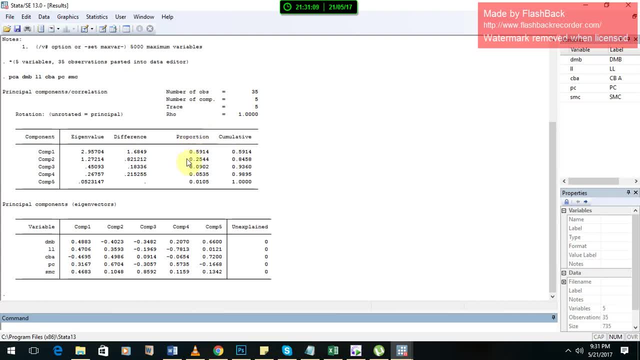 So Here you can see that the First components showing almost 60% of variation- this is the first component out of five components- and the second component is showing almost 25, and the rest of them are showing pretty much less variation. so, based on the eigen, 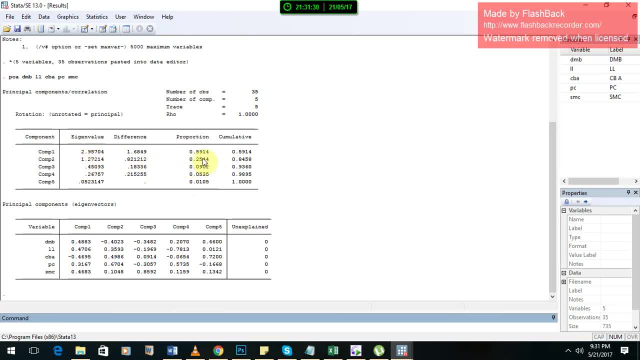 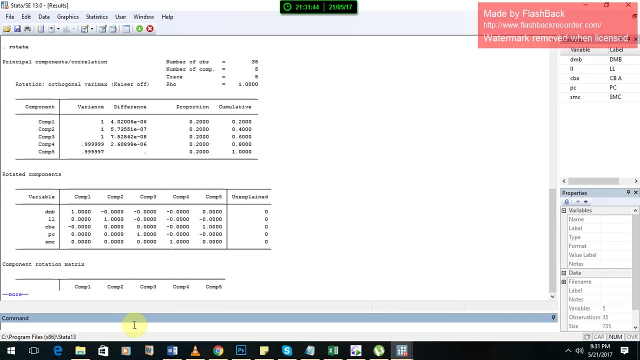 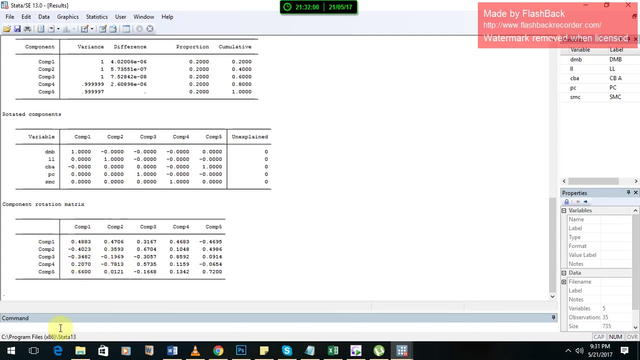 values, usually greater than 1, are selected, so it might create an index using first two components. then we have to write the command to rotate, rotate, press, Enter what it will give you. it gives you the orthogonal value max. it gives you the variation of each variable in each component. so then we are going. 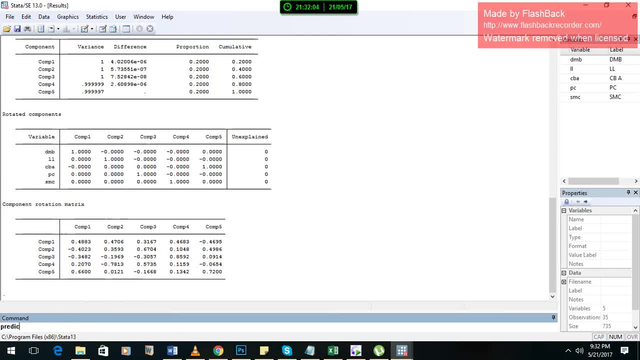 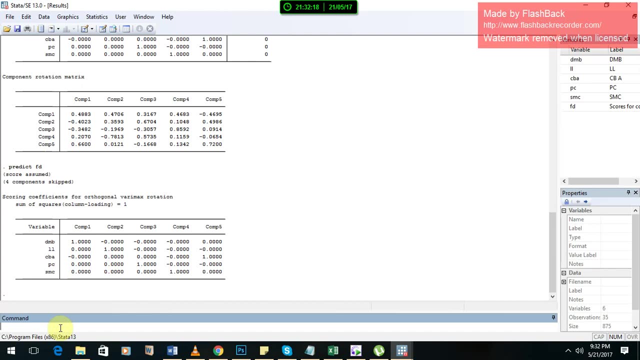 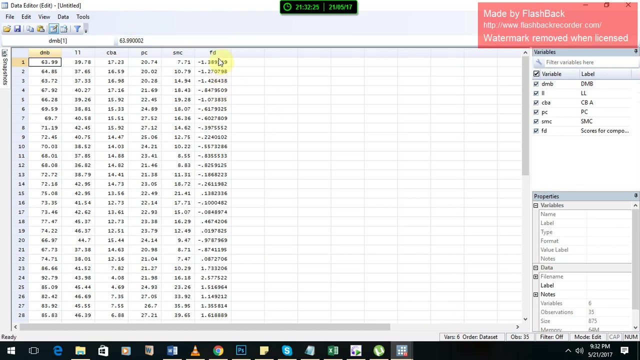 to finally write over here: predict and space and whichever the variable you want to name for my financial draft index. I'm going to write FD, so I'm going with FD. press enter now. after predict, you will go to the data window and there you will see that a sixth column. this is the 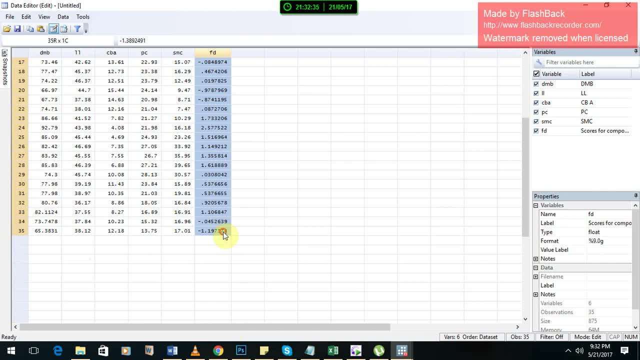 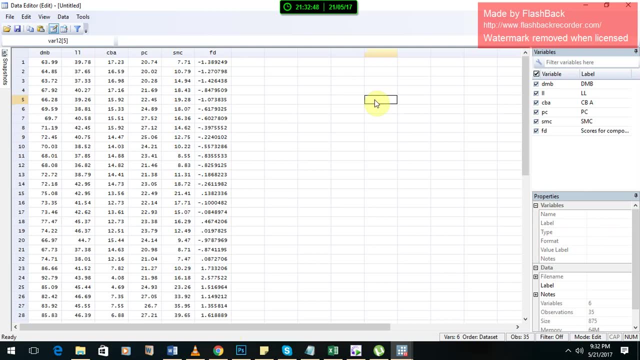 final index. these values you can use in your regression or wherever you want to choose it as your final index. so that's pretty much it. thanks for watching. please subscribe for more videos, thank you.